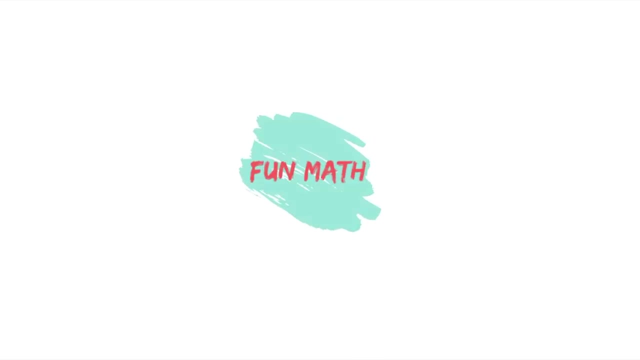 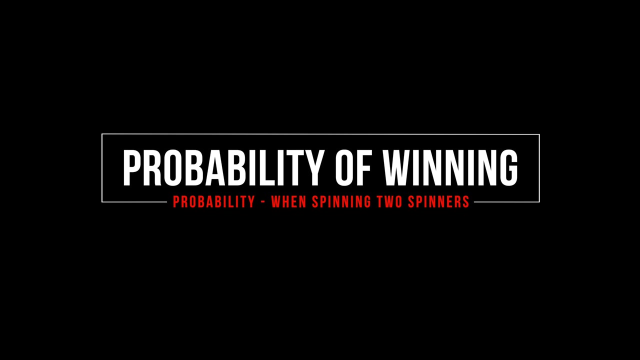 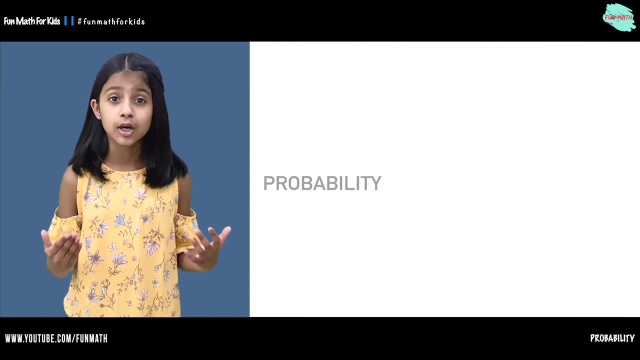 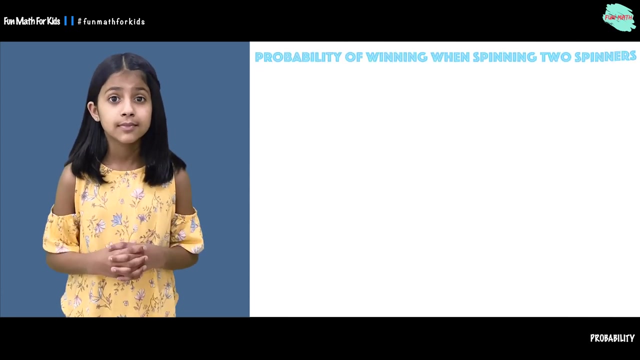 Welcome to Fun Math. Today we will be continuing talking about probability. You will see the probability of winning when spinning two spinners. Two spinners are spun. You win when you get the same color on both spinners. Let's find out the probability of winning. Here we have. 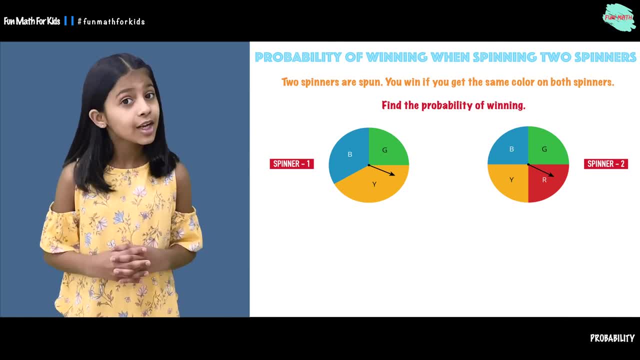 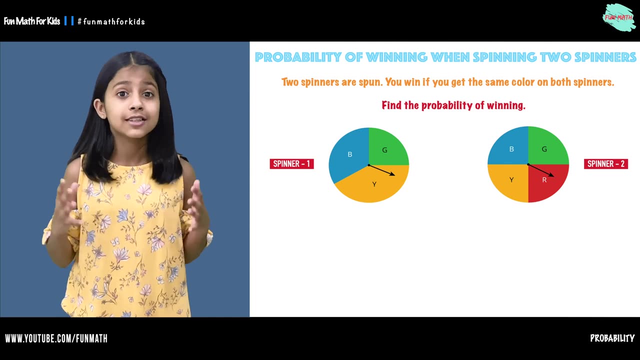 two spinners: Spinner one and spinner two. On spinner one, we have three colors: Blue, green and yellow. On spinner two, we have four colors: Blue, green, red and yellow. So here we have a game To win. you need to get the same color on both spinners. So how many? 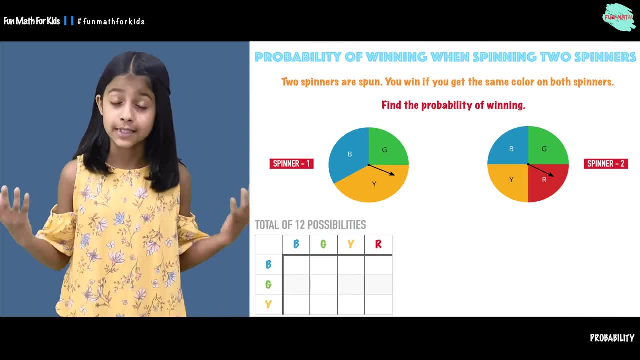 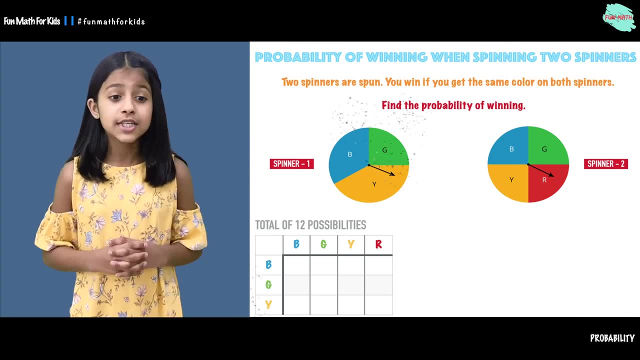 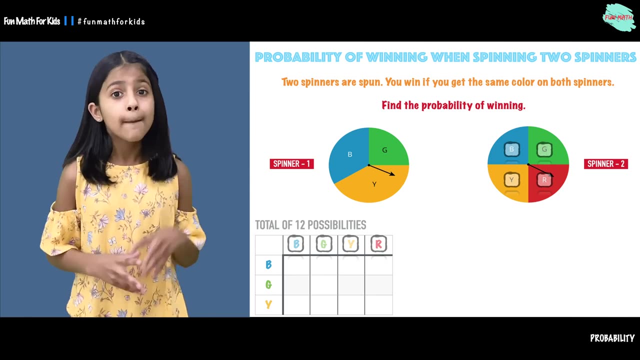 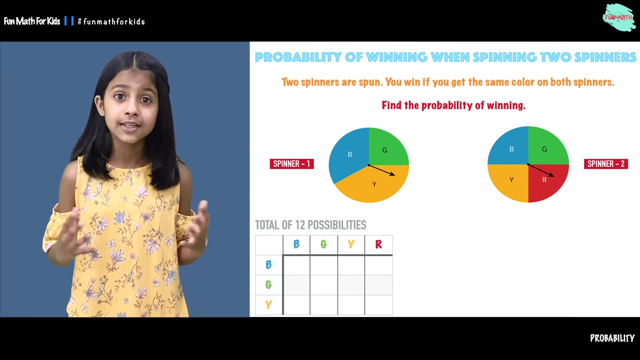 possibilities are there. There are 12 total possibilities. So in this table we have spinner one which is blue, green and yellow And we have spinner two which is blue, green, yellow and red. How many possibilities are there of winning? There are three possibilities. 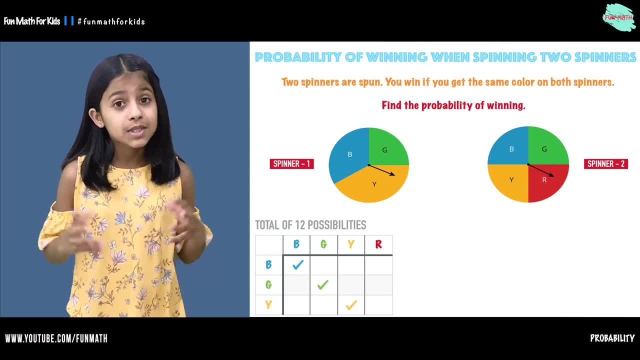 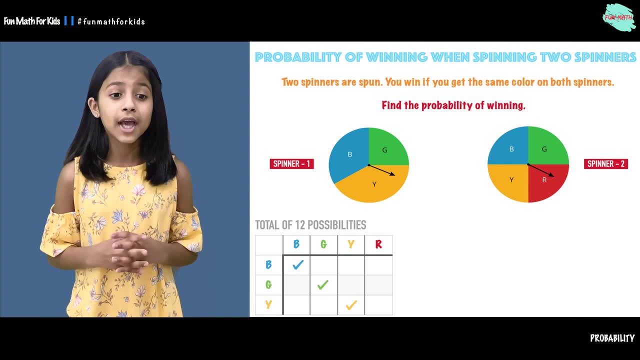 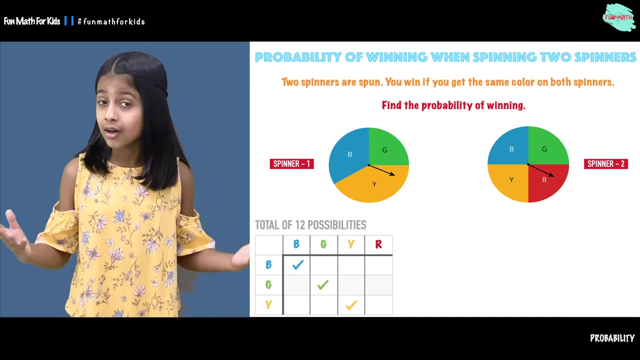 Let's see how There are three possibilities, because on spinner one we have one blue. That's why we have blue, And on spinner two we have also another blue. That is why we have. that is why blue and blue is one possibility. Similarly with green and green and yellow and yellow, If you get. 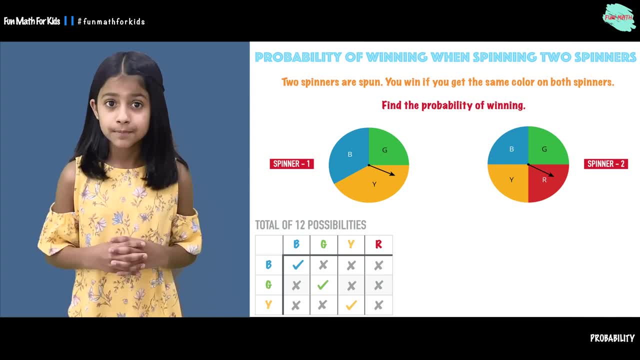 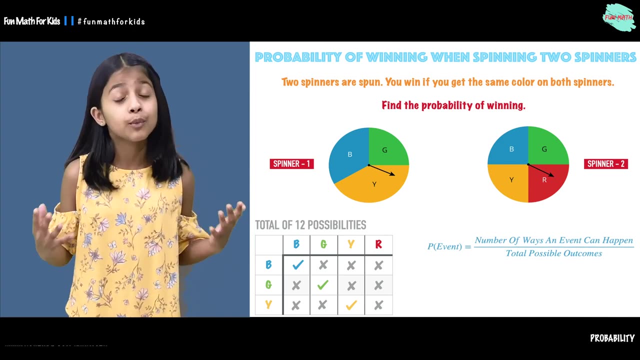 on the rest of the possibilities, you will lose the game. So now let's talk about what is the probability of winning. Before we move on to that, let's first talk about the formula. The formula is the probability of an event, is the number of ways an event can happen over the total possible outcomes. 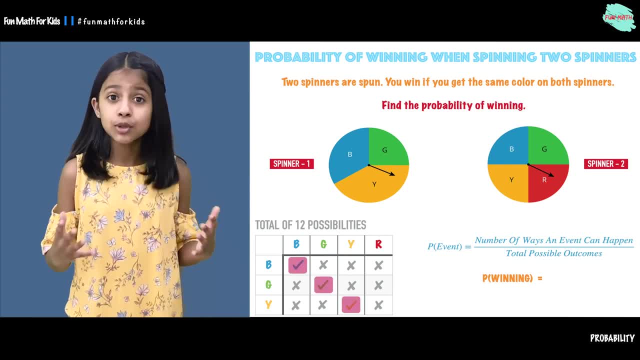 The probability of winning is three as our numerator, because there are three ways of winning Right on the table. And what is our denominator? Our denominator has to be 12 because there are 12 total possibilities. So what is our denominator? Our denominator has to be 12 because there are 12 total possibilities. 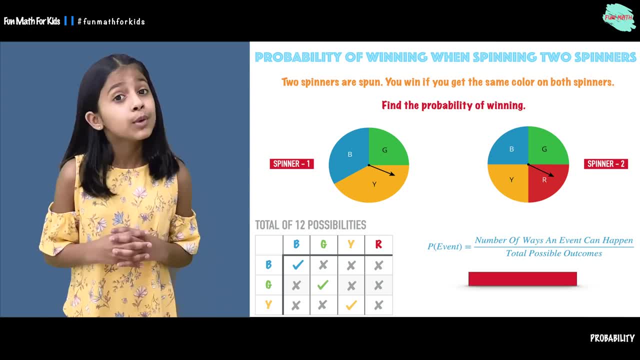 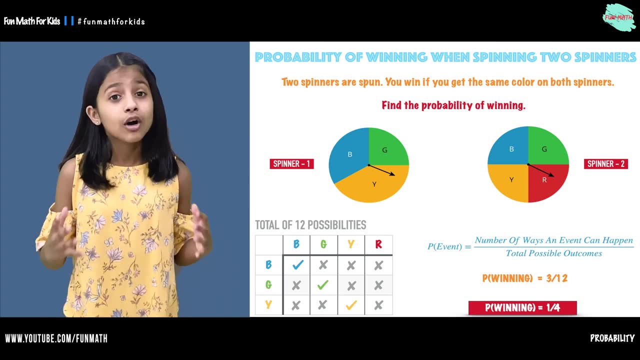 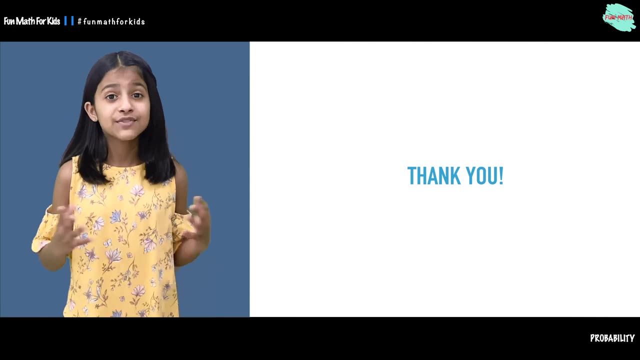 That is why we have 3 over 12.. If we reduce this fraction we will get the probability of winning is 1 over 4.. This can also be said as the probability of winning is 25 percent. That is all for now. Thanks for watching. 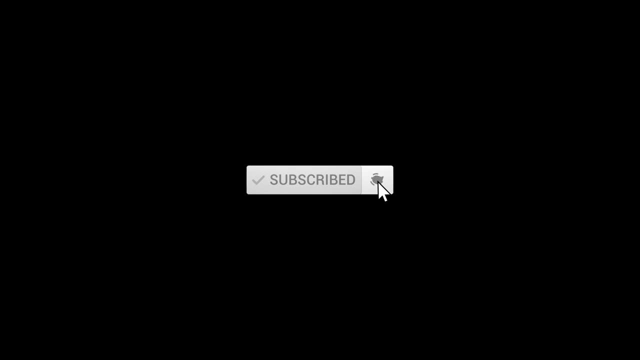 We will see you in the next video. 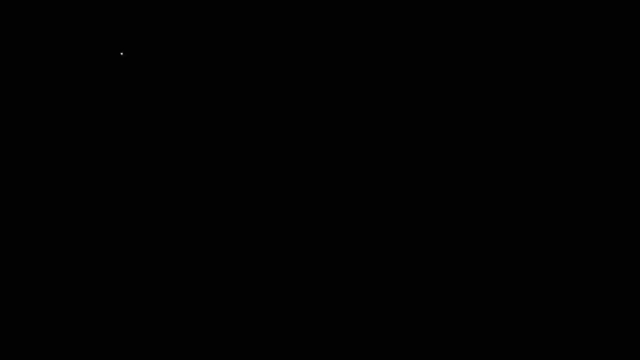 In this video we're going to focus on trigonometric integrals, But now to begin, you may want to write down some notes just to review some formulas that will be useful when integrating trigonometric expressions. First, sine squared plus cosine squared- you need to know that equals 1.. 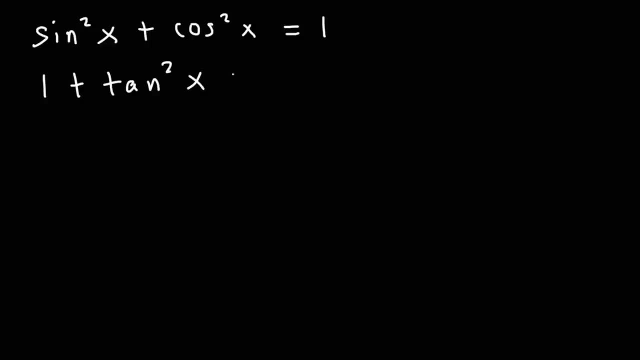 Next, 1 plus tangent squared is equal to secant squared. This is a good review of some trigonometric formulas that you've been exposed to in the past. The next one you need to be familiar with is: 1 plus cotangent squared is equal to cosecant squared. 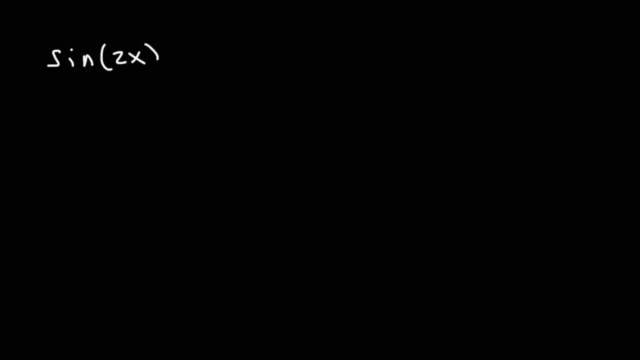 Next we have the double angle formulas: Sine 2x is equal to 2 sine x, cosine x And then cosine 2x. there's three forms that you can convert this into. You can convert it to cosine squared. You can set it equal to 1 minus sine squared. 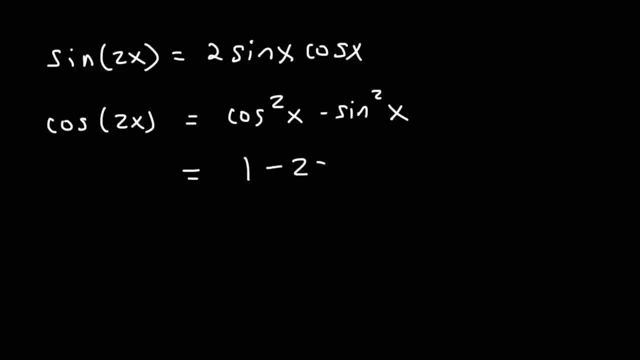 You can set it equal to 1 minus 2 sine squared Or 2 cosine squared minus 1.. Next up are the power reducing formulas. Sine squared can be reduced to 1 half 1 minus cosine 2x, And cosine 2x can be reduced to 1 half 1 minus cosine 2x. 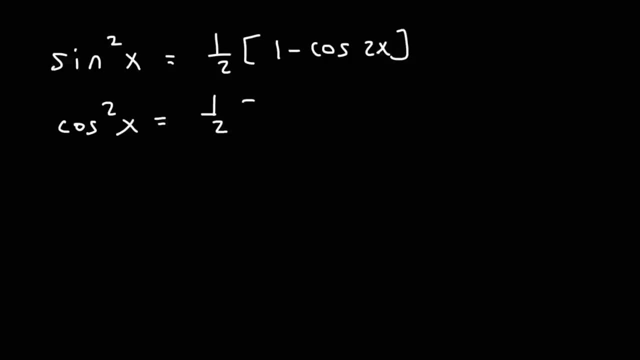 Sine squared can be reduced to 1 half 1 plus cosine 2x, And you can reduce that to 1 half 1 plus cosine 2x. Sine is equal to cosine squared. Now there are some other trigonometric formulas that you may need to know, which I'll introduce later in. 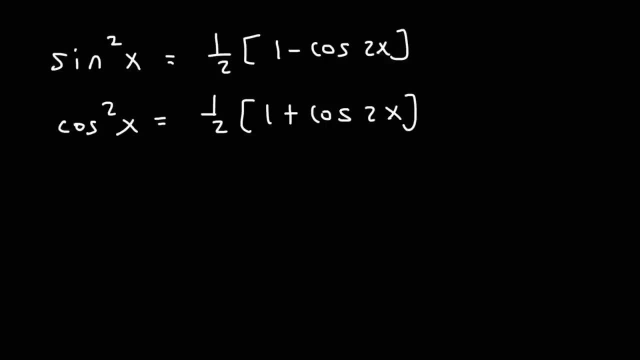 this video when it becomes relevant, But for now we can work with what we have here. So let's go to cosine, to the third x. Now, the first problem that we're going to work on is this one: Let's find the anti derivative of cosine to the third x.